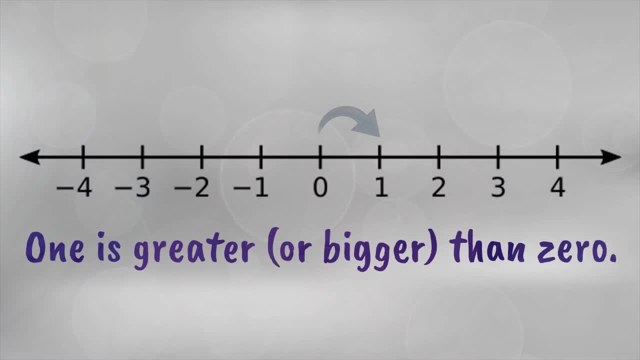 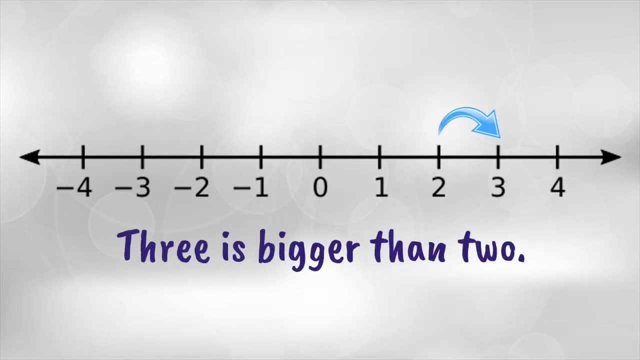 I mean no pancakes, that would be so sad. One is greater or bigger than zero. Two is bigger than one. Three is bigger than two. Four is bigger than three. You get the idea. Now, if we move the opposite direction on the number line, every number gets smaller. 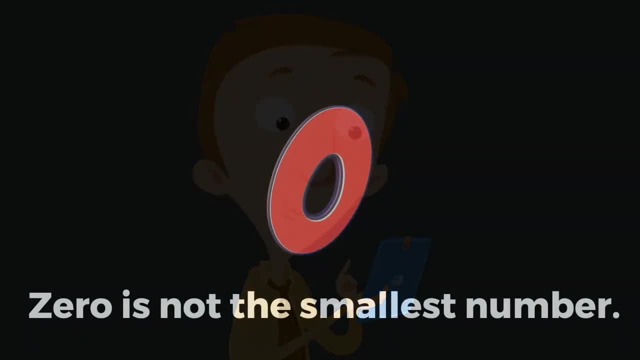 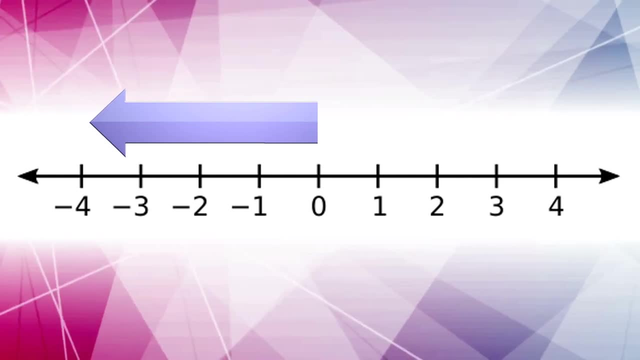 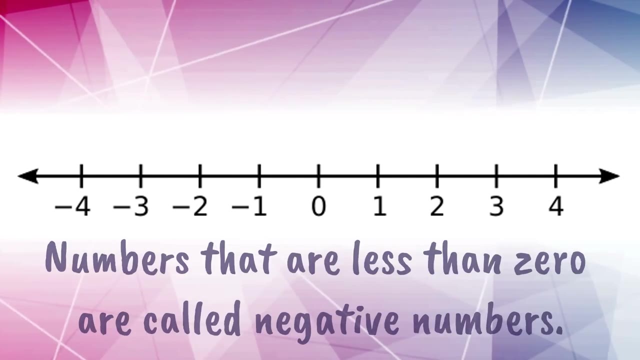 Yeah, Now here's something interesting: Zero is not the smallest number. Numbers can go lower than zero. I mean zero is in the middle of this number line, which means all of these numbers are less than zero. Numbers that are less than zero are called negative numbers. 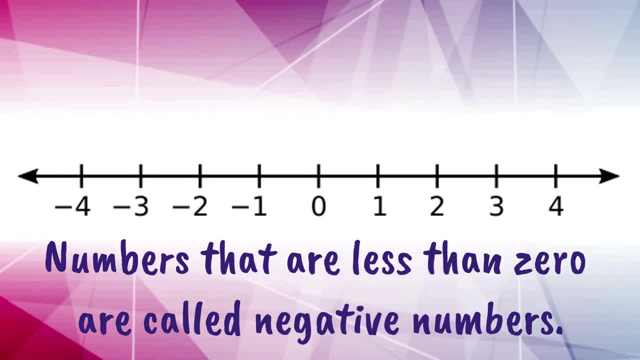 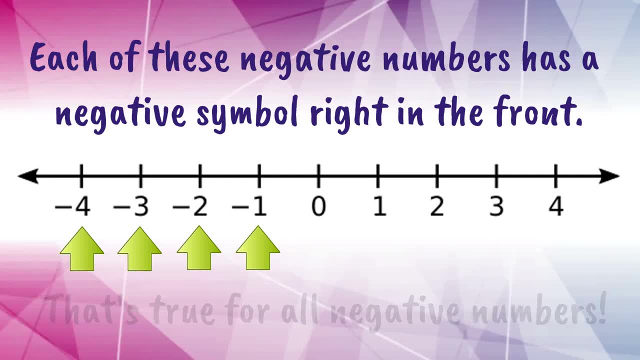 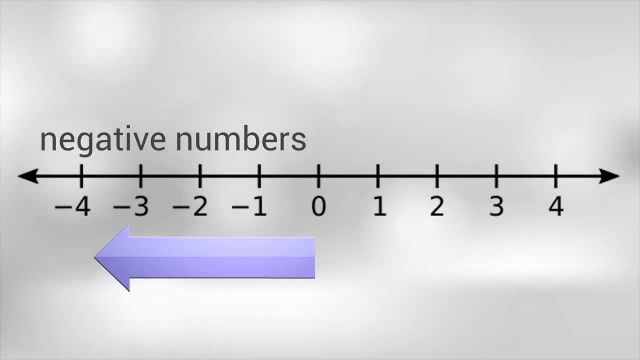 Negative numbers. Negative numbers- That's what they are. Now, you might have noticed, each of these negative numbers has a negative symbol right in front. That's true for all negative numbers, so they're really easy to spot. So numbers that are less than zero are called negative numbers, which makes sense. 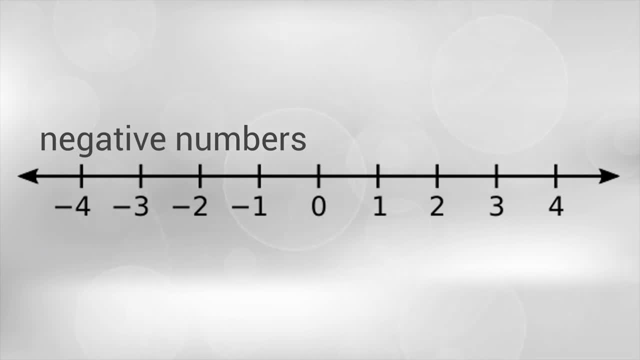 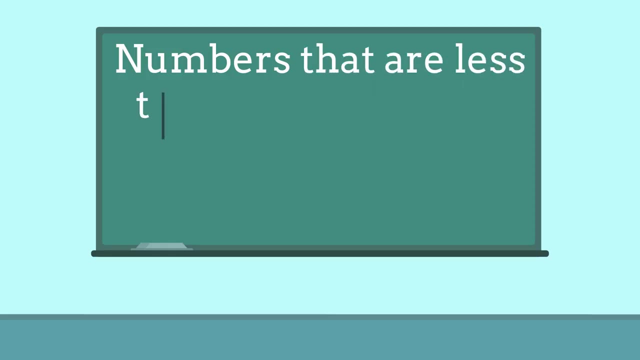 They have this negative sign in front of them. Numbers that are greater than zero are called positive numbers. Yeah, positive numbers. They are easy to spot too. Just look for numbers that don't have a negative sign in front of them. So numbers that are less than zero are called negative numbers, which makes sense. 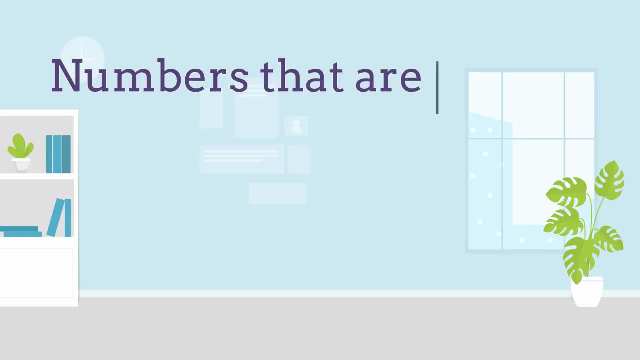 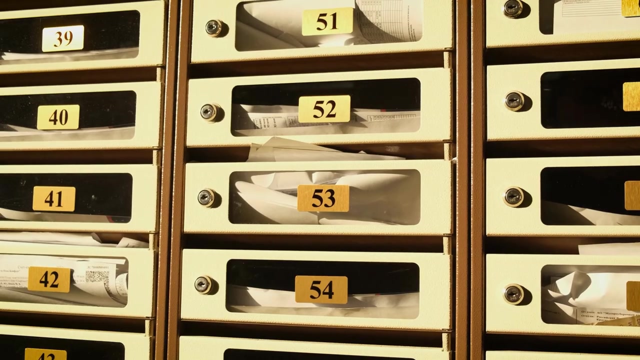 They have this negative sign in front of them. Numbers that are greater than zero are called positive numbers. Yeah, positive numbers. They are easy to spot too. Just look for numbers that don't have a negative sign in front of them. Let's talk a little bit more about positive numbers. 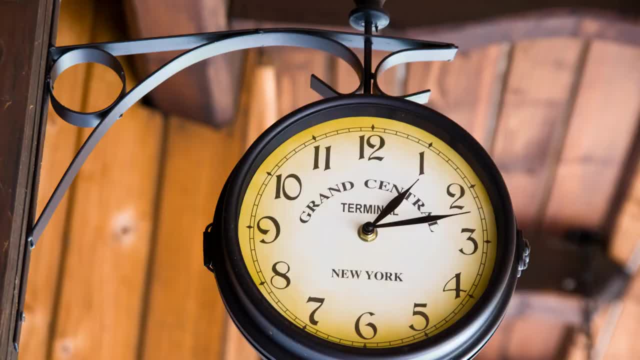 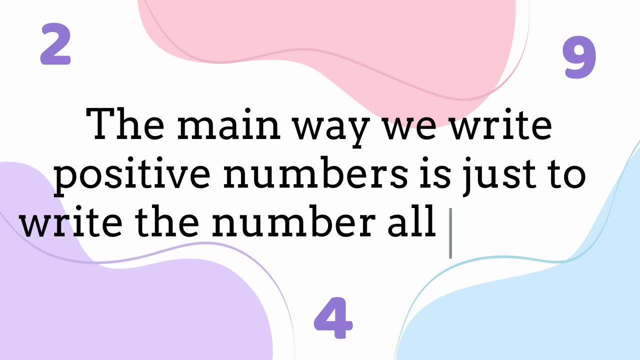 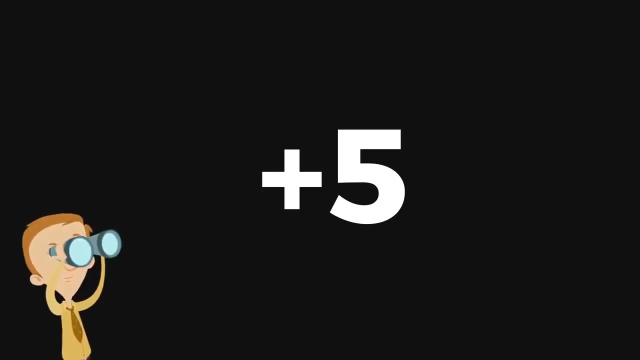 Positive numbers are very common, Very common. We see them everywhere. So much so that the main way we write positive numbers is just to write the number all by itself. You can put a positive sign in front of a positive number if you'd like, but you don't have to. 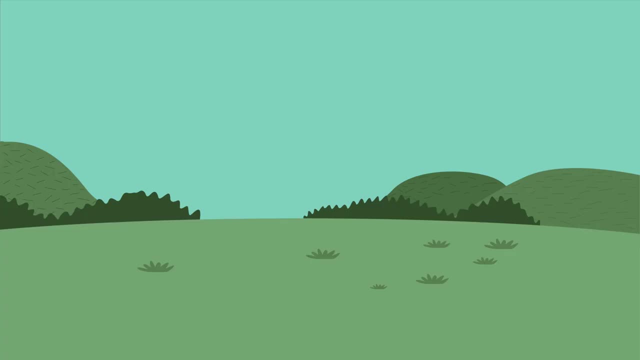 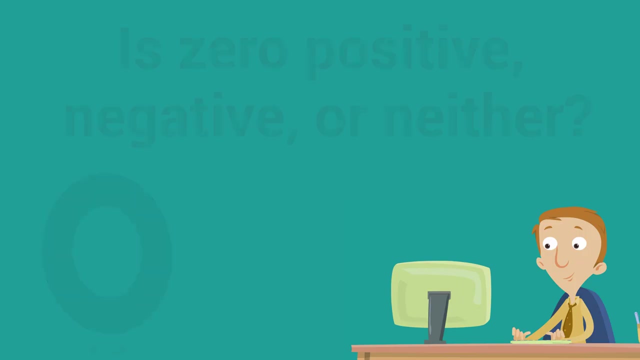 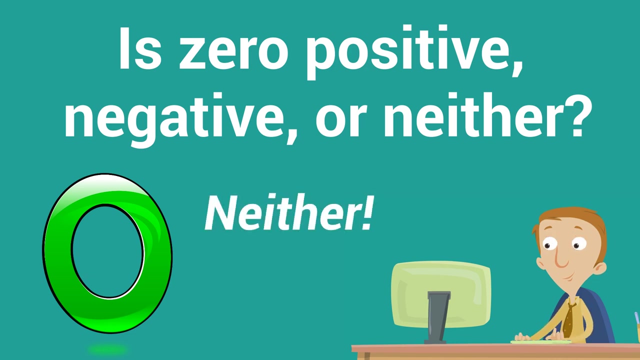 Most of the time, it's just the number. Positive numbers, Negative numbers, Pretty simple. Wait, what about zero? Is zero positive, negative or neither? Well, neither Zero is actually the only number that isn't positive or negative. 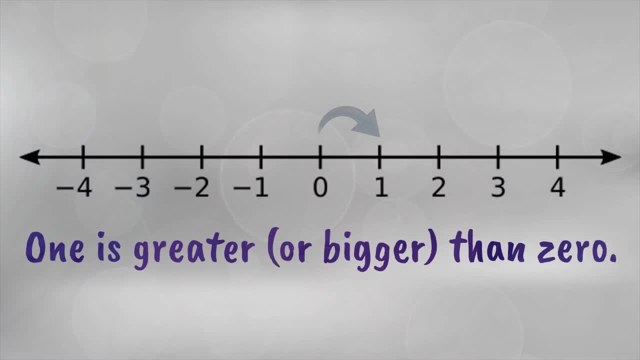 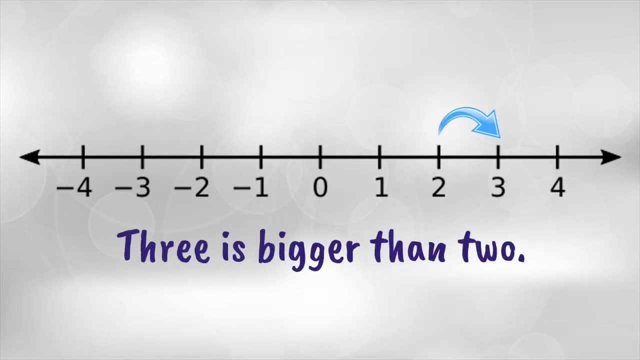 I mean no pancakes, that would be so sad. One is greater or bigger than zero. Two is bigger than one. Three is bigger than two. Four is bigger than three. You get the idea. Now, if we move the opposite direction on the number line, every number gets smaller. 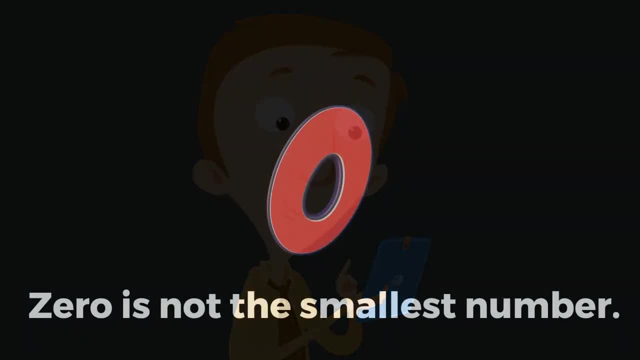 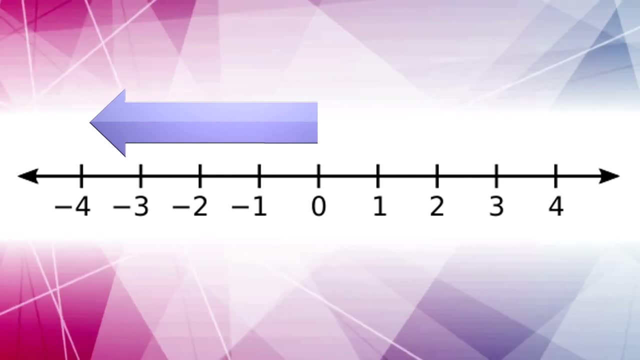 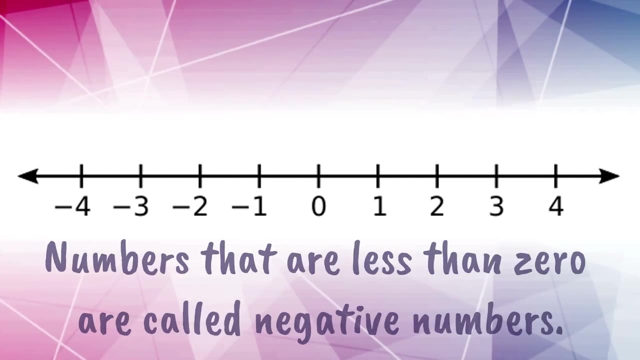 Yeah, Now here's something interesting: Zero is not the smallest number. Numbers can go lower than zero. I mean zero is in the middle of this number line, which means all of these numbers are less than zero. Numbers that are less than zero are called negative numbers. 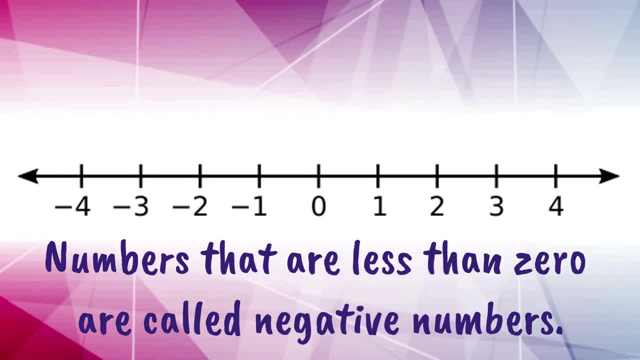 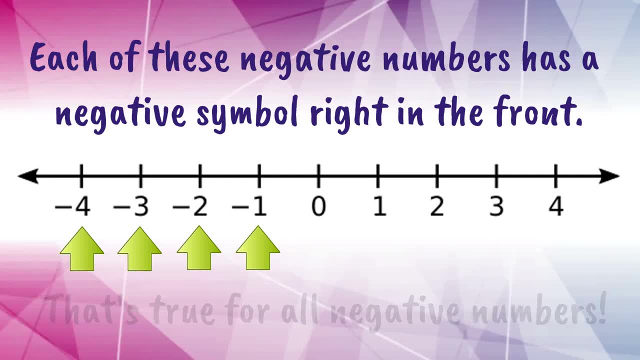 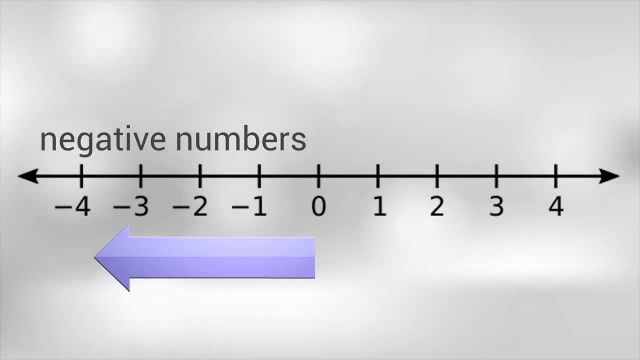 Negative numbers. Negative numbers- That's what they are. Now, you might have noticed, each of these negative numbers has a negative symbol right in front. That's true for all negative numbers, so they're really easy to spot. So numbers that are less than zero are called negative numbers, which makes sense. 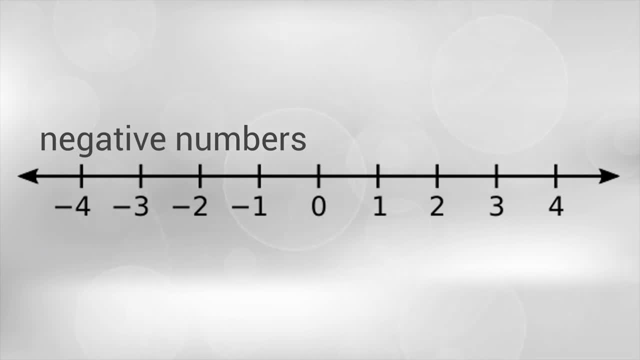 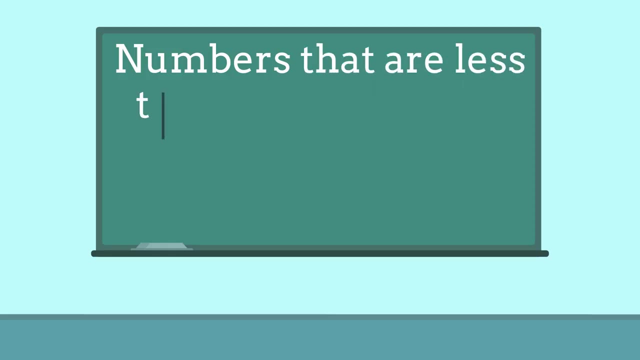 They have this negative sign in front of them. Numbers that are greater than zero are called positive numbers. Yeah, Positive numbers. They are easy to spot too. Just look for numbers that don't have a negative sign in front of them. So numbers that are less than zero are called negative numbers, which makes sense. 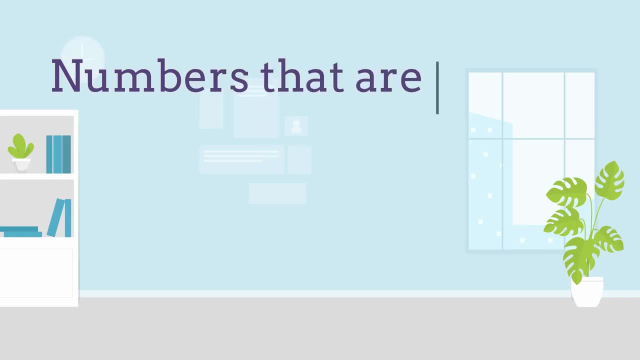 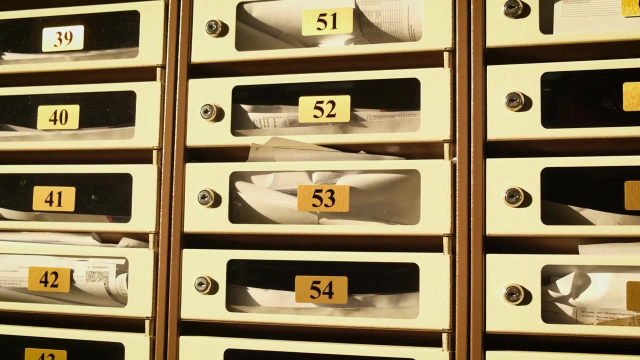 They have this negative sign in front of them. Numbers that are greater than zero are called positive numbers. Yeah, Positive numbers. They are easy to spot too. Just look for numbers that don't have a negative sign in front of them. Let's talk a little bit more about positive numbers. 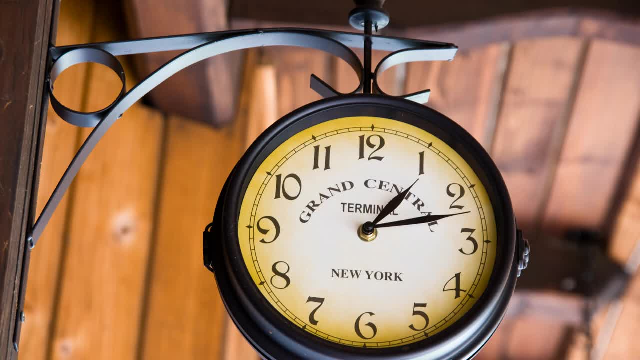 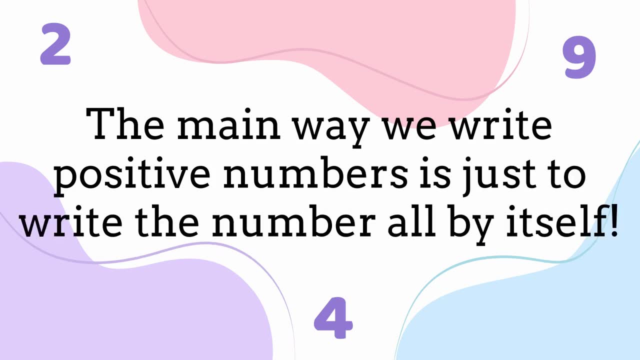 Positive numbers are very common, Very common. We see them everywhere. So much so that the main way we write positive numbers is just to write the number all by itself. You can put a positive sign in front of a positive number if you'd like, but you don't. 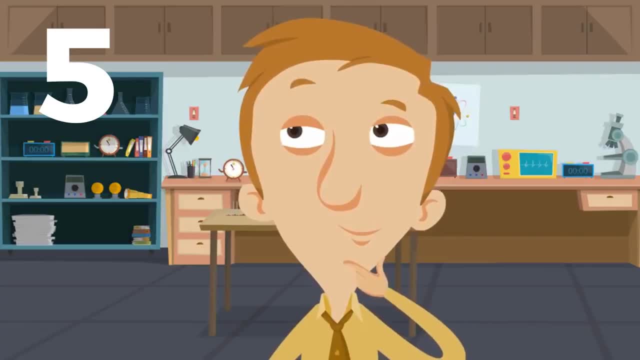 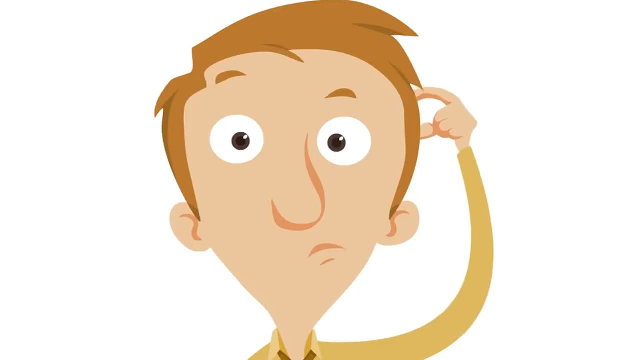 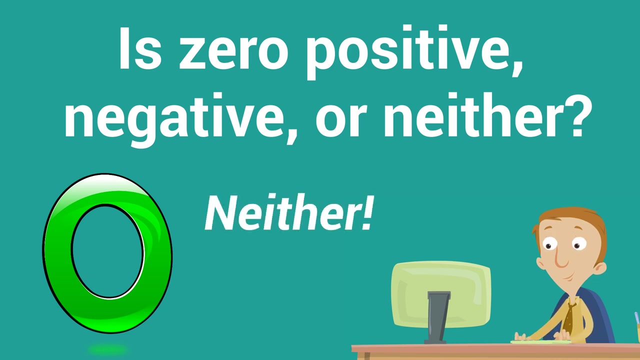 have to. Most of the time, it's just the number: Positive numbers, negative numbers, Pretty simple. Wait, what about zero? Is zero positive, negative or neither? Well, neither Zero is actually the only number that isn't positive or negative. 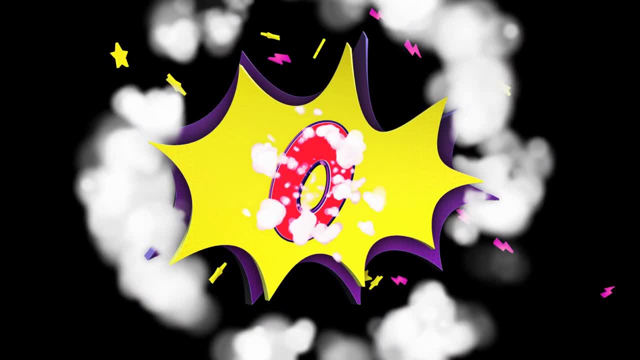 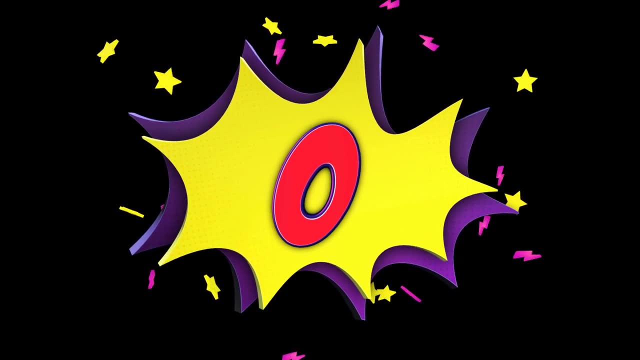 It's kind of in the middle of all of them in its own category, Zero. It isn't positive or negative, It's, you know, zero. Hey, we use positive numbers a lot, right, We see them all around us. 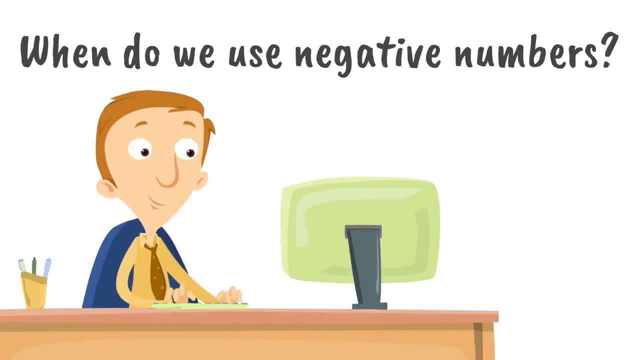 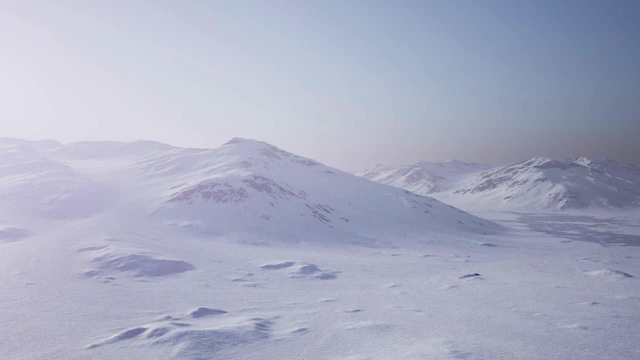 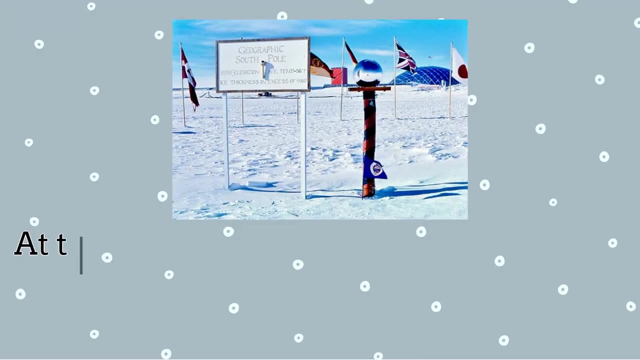 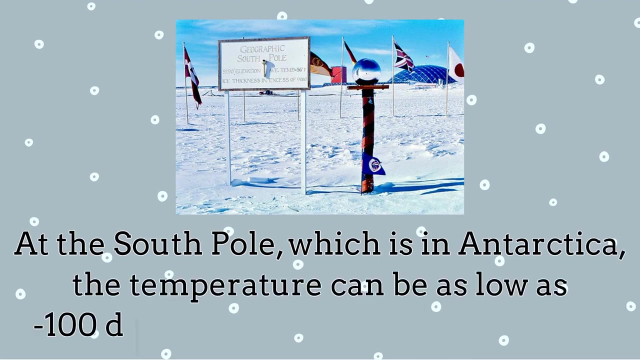 But when do we use negative numbers, Numbers that are less than zero? Check this out. This is footage from Antarctica, the fifth largest continent in the world. What do you think the temperatures are like there? Yeah, super cold. At the South Pole, which is in Antarctica, the temperature can be as low as negative. 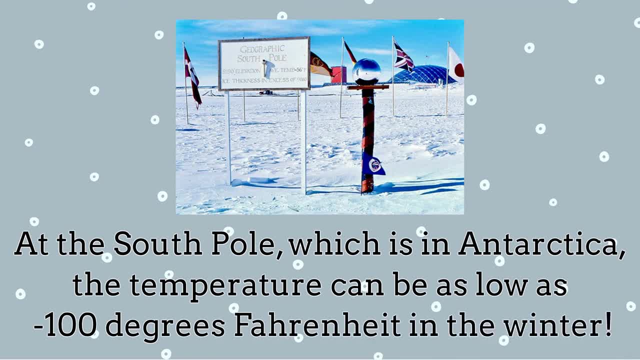 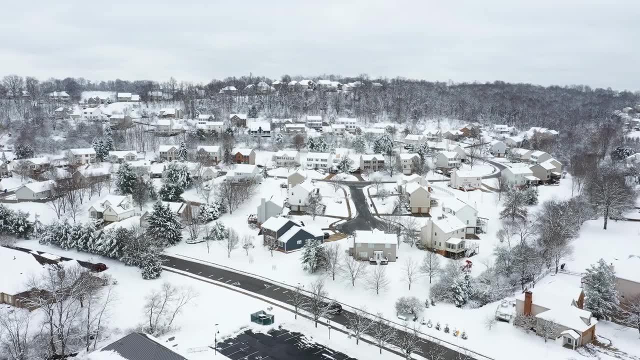 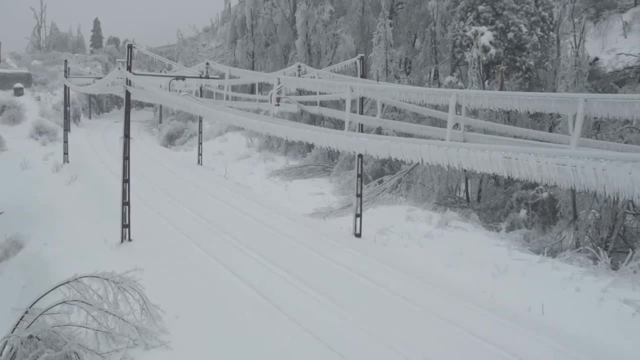 100 degrees Fahrenheit in the world. It's like you know, the temperature is like negative 100 degrees Fahrenheit in the winter, Negative 100 degrees, Wow. If you live in an area that gets really cold temperatures, maybe you've experienced how 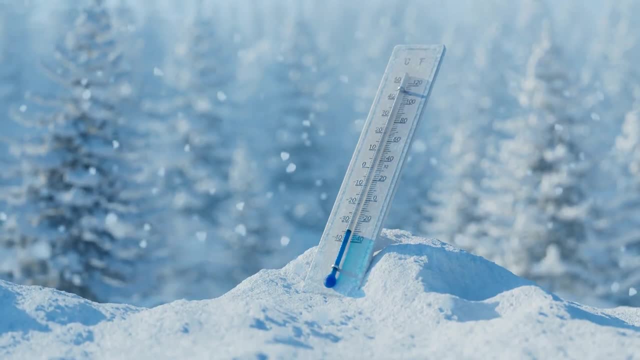 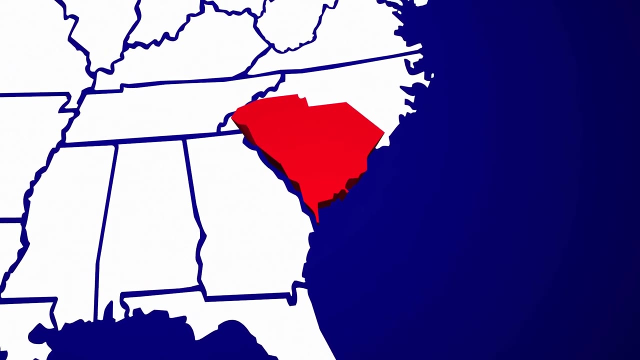 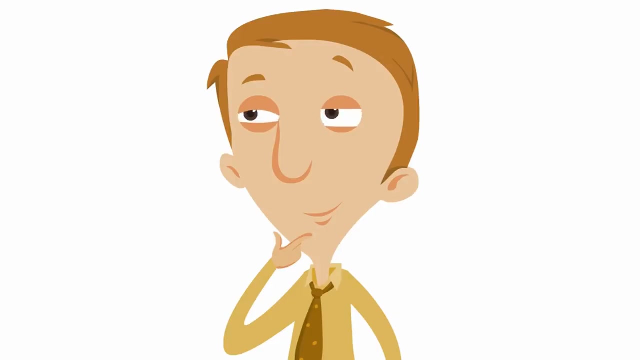 cold. it is when the temperature reaches negative degrees. negative numbers- Wow Numbers so low, they dip below zero. Me, I'm always in positive numbers here. I don't know what negative temperatures feel like, I can only imagine. Another example of negative numbers is when we look at the elevation of different places. 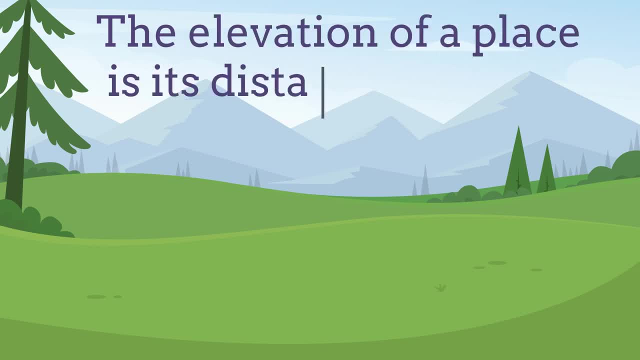 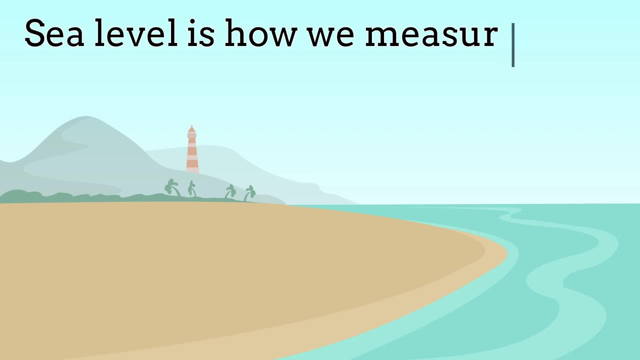 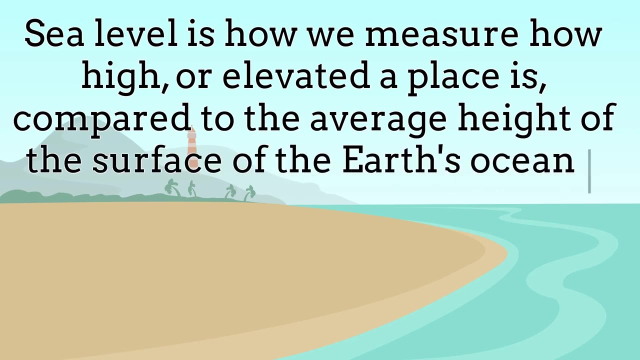 on Earth. The elevation of a place is its distance above or below sea level. Now, what's sea level? Well, sea level is how we measure how high or elevated a place is compared to the average height of the surface of the Earth's oceans. 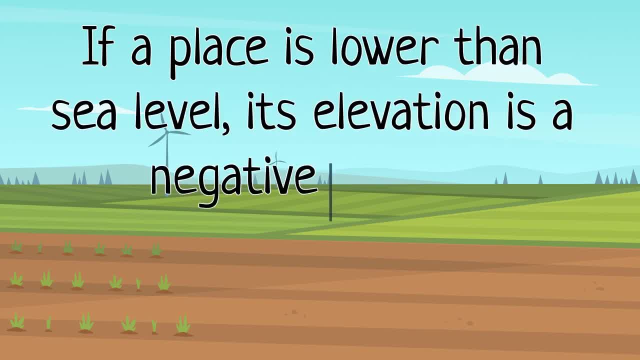 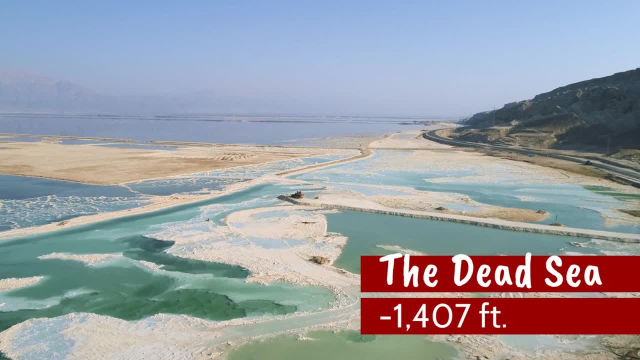 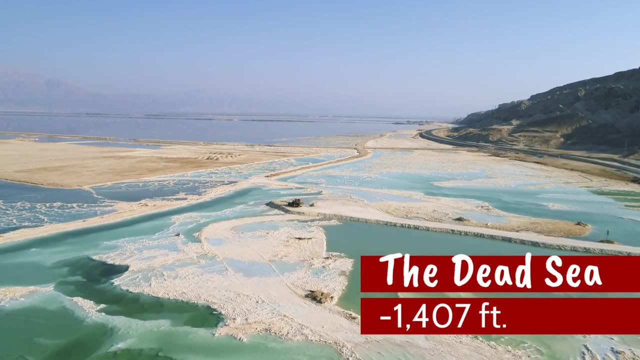 Now, if a place is lower than sea level, its elevation is a negative number. For example, a place called the Dead Sea is at negative 1,407 feet- Negative 1,407 feet. In North America there's a place called Badwater Basin. 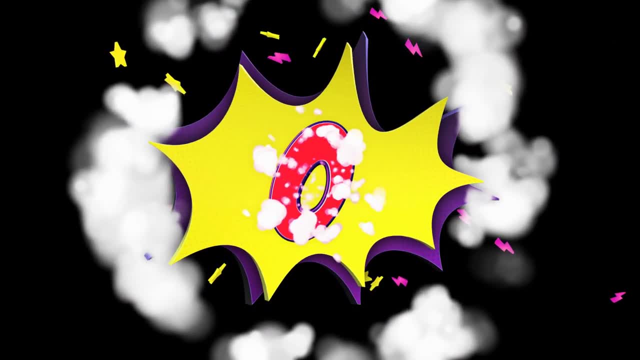 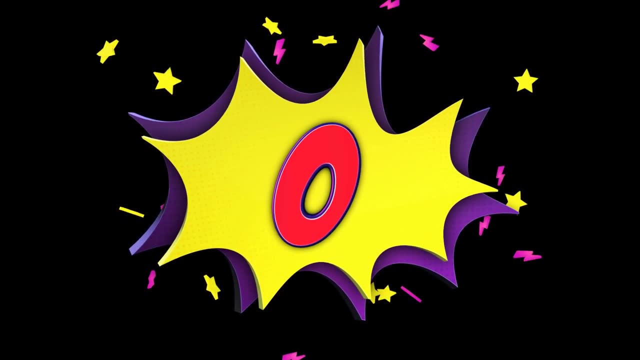 It's kind of in the middle of all of them in its own category, Zero. It isn't positive or negative, It's, you know, zero. Hey, we use positive numbers a lot, right, We see them all around us. 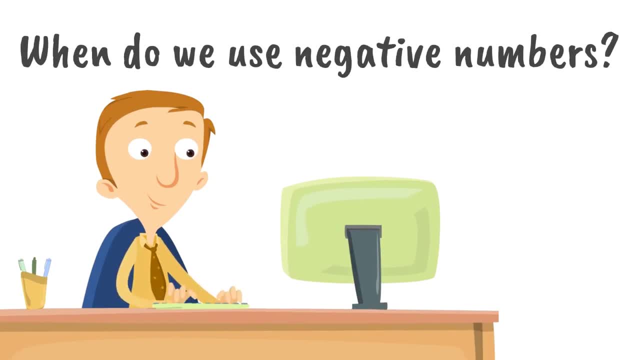 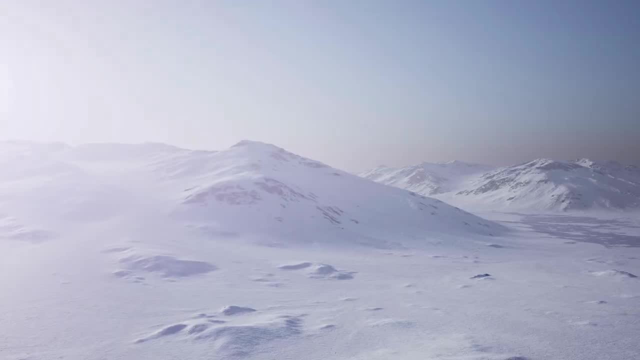 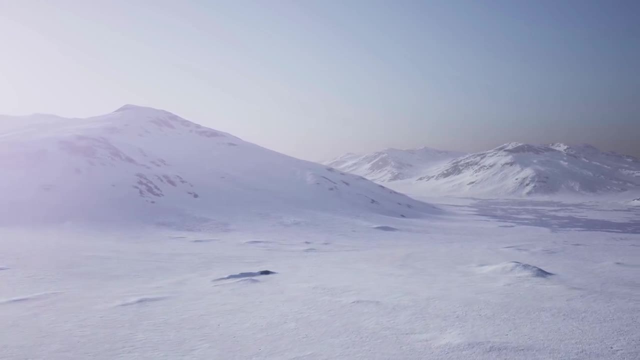 But when do we use negative numbers, Numbers that are less than zero? Check this out. This is footage from Antarctica, the fifth largest continent in the world. What do you think the temperatures are like there? Yeah, super cold At the South Pole, which is in Antarctica. 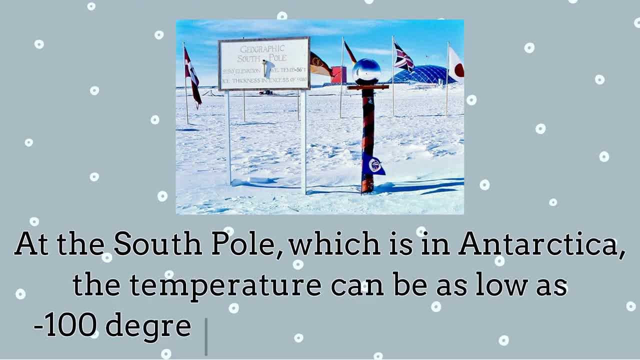 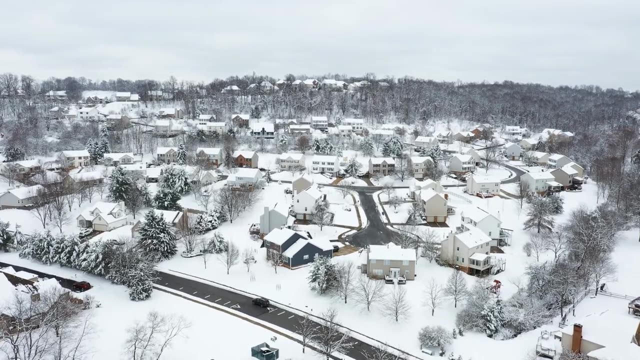 the temperature can be as low as negative 100 degrees Fahrenheit. 100 degrees Fahrenheit in the winter, Negative 100 degrees- Wow. If you live in an area that gets really cold temperatures, maybe you've experienced how cold it is when the temperature reaches negative degrees, negative numbers. 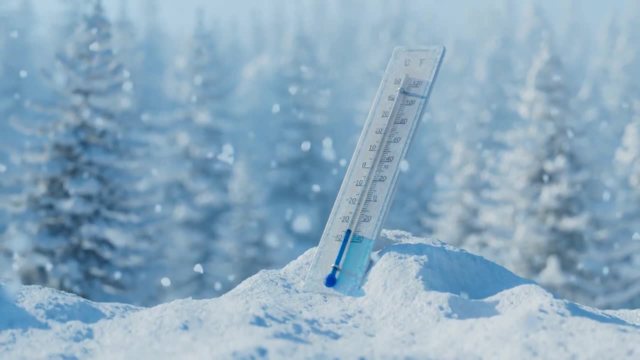 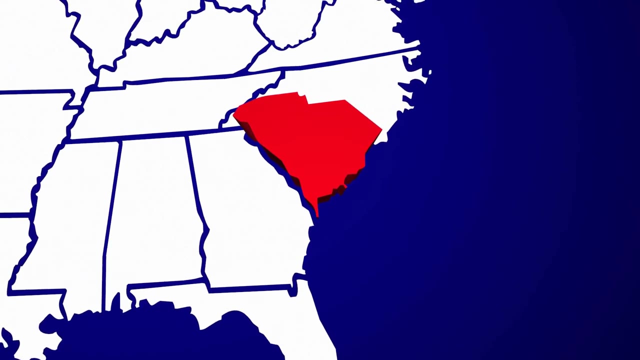 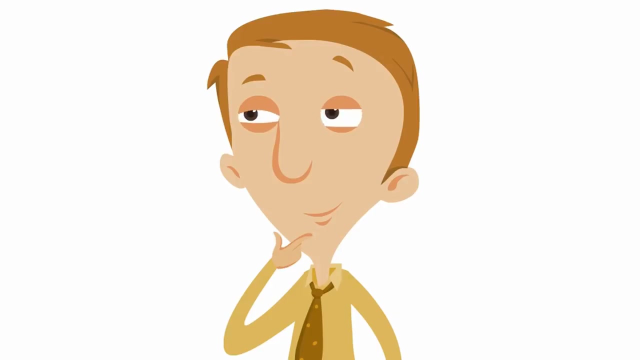 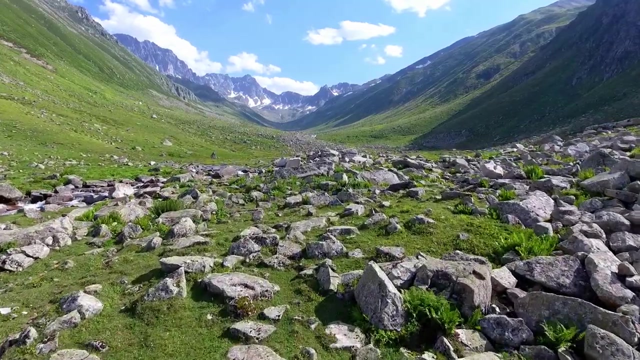 Wow, Numbers so low. they dip below zero. Me, I live in South Carolina, So, yeah, the temperature is always in positive numbers here. I don't know what negative temperatures feel like, I can only imagine. Another example of negative numbers is when we look at the elevation of different places on Earth. 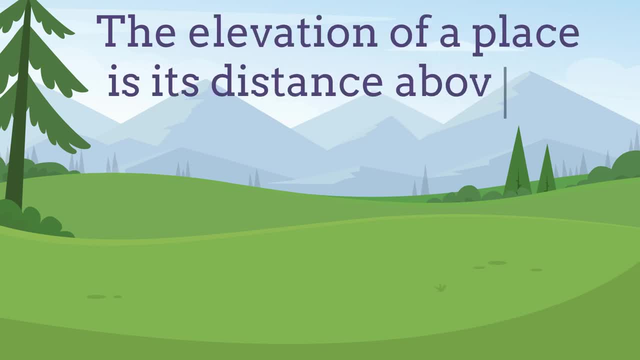 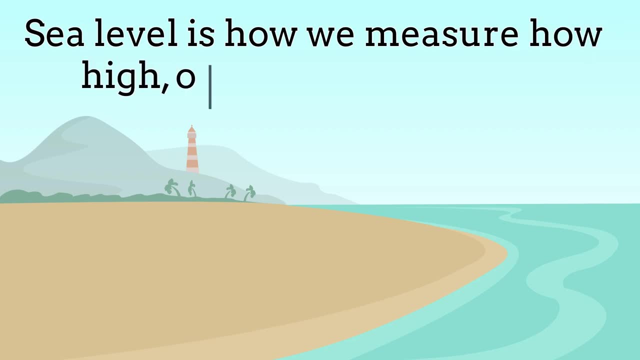 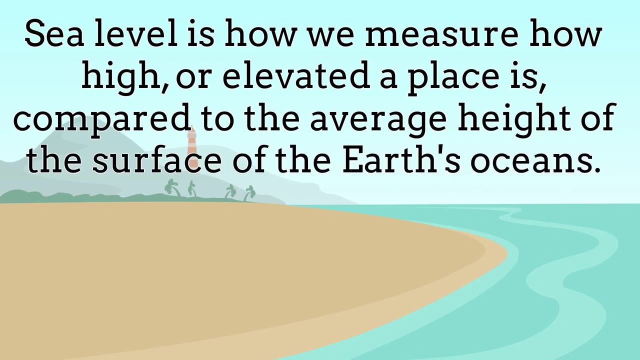 The elevation of a place is its distance above or below sea level. Now, what's sea level? Well, sea level is how we measure how high or elevated a place is compared to the average height of the surface of the Earth's oceans. Now, if a place is lower than sea level, 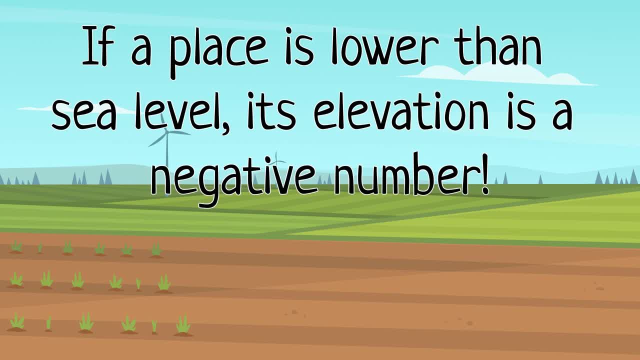 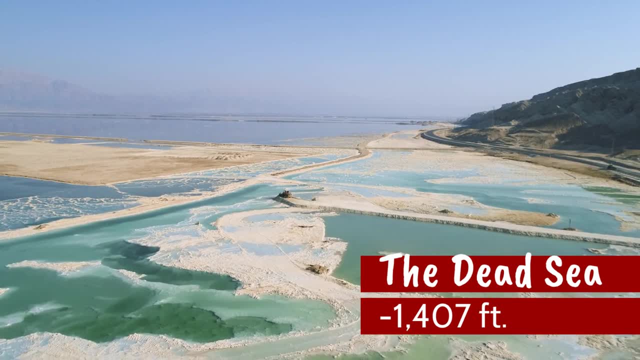 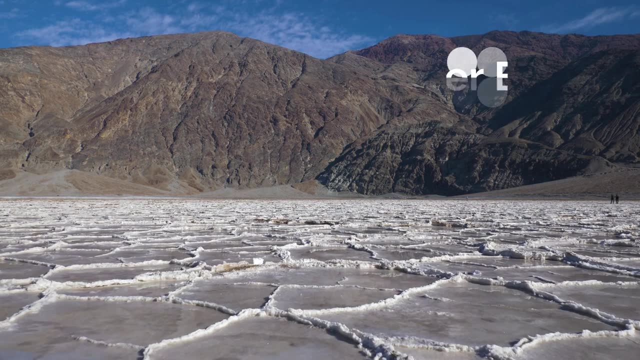 its elevation is a negative number. For example, a place called the Dead Sea is at negative 1,407 feet, Negative 1,407 feet. In North America there's a place called Badwater Basin- Badwater Basin. If you are at Badwater Basin, 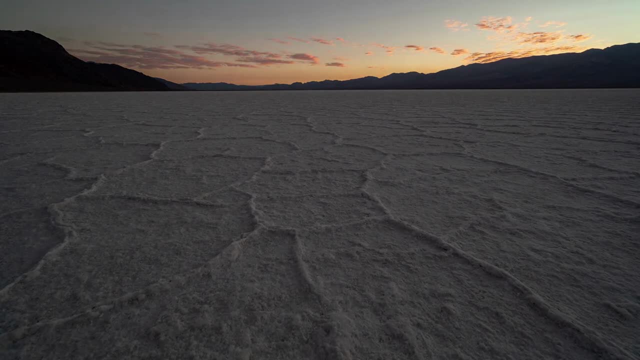 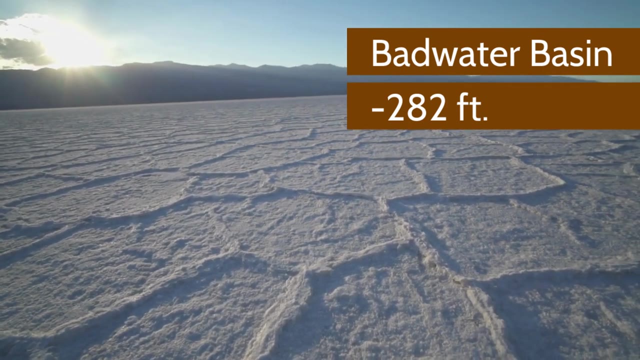 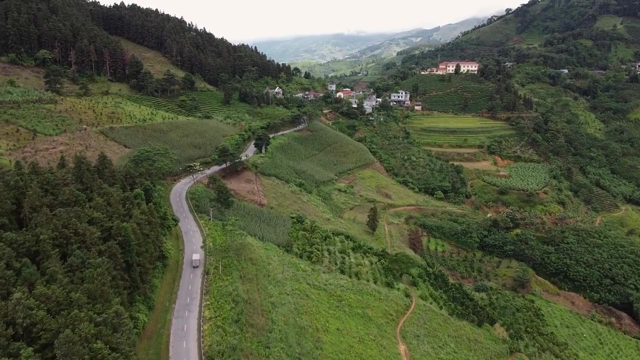 Badwater Basin. If you are at Badwater Basin, you are at negative 282 feet. That means you are 282 feet below sea level. Of course, elevations can be positive numbers and most places on land are above sea level. 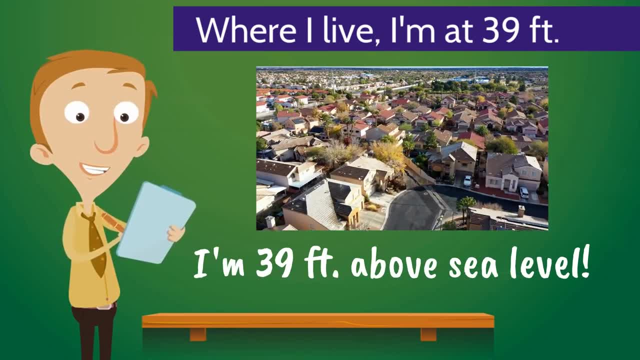 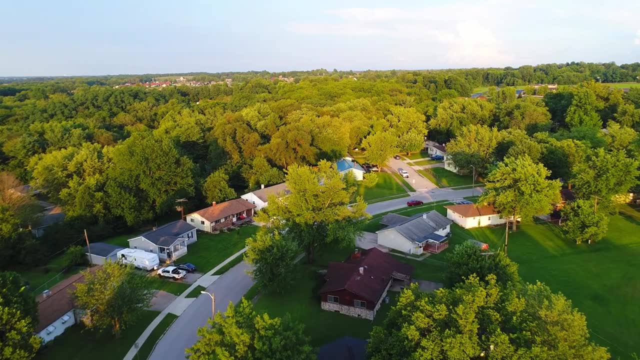 Where I live, I'm at 39 feet, meaning I'm 39 feet above sea level. If you're curious about what the elevation is, check out this video. It's called Badwater Basin. The elevation is where you live. You can ask a parent or teacher. 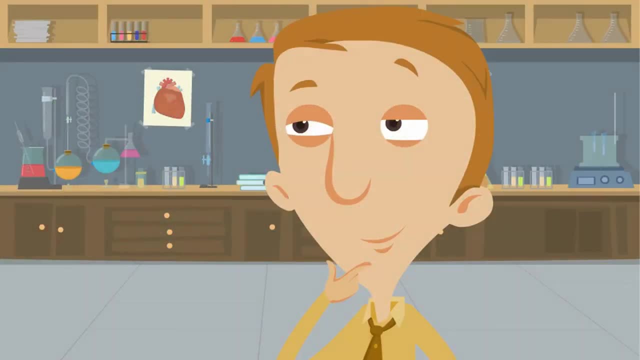 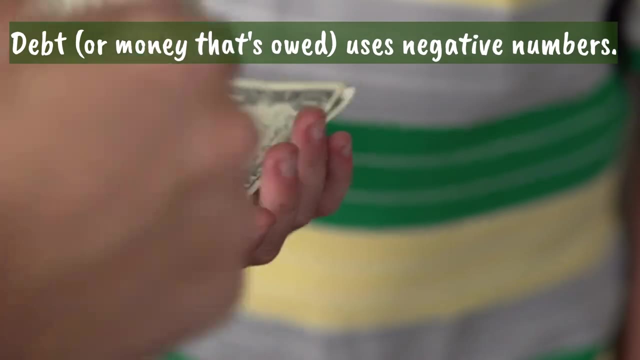 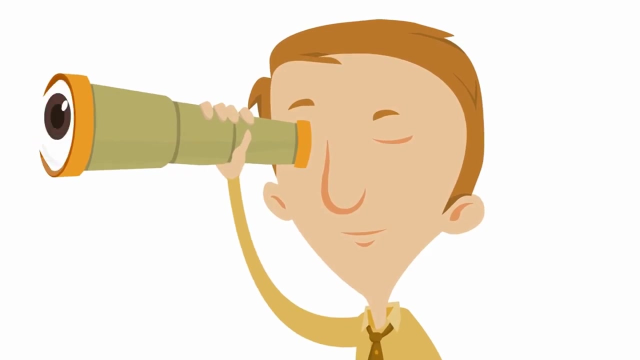 It's kind of fun to find out, Alright. the last example of negative numbers is if you owe someone money, Debt or money that's owed, uses negative numbers. For money you get, you would use positive numbers. Okay, you know what? 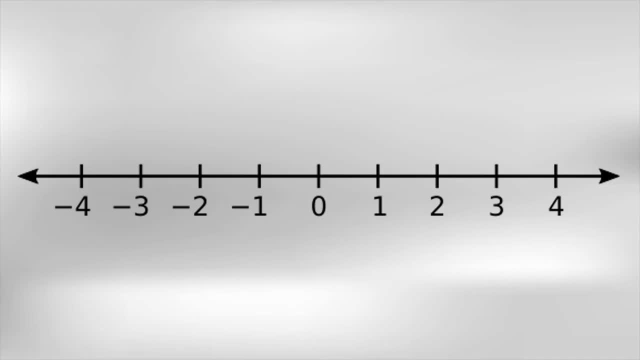 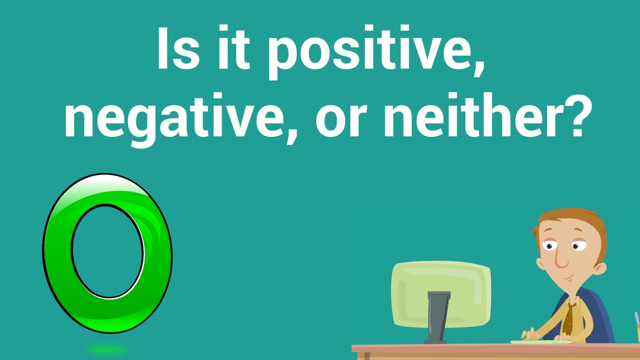 It's time to review. It's time to review. Numbers below zero are called Yeah, Negative, Yeah, Negative numbers, Great job. Numbers above zero are called Got it Positive numbers, Positive numbers, Awesome And zero. Is it positive, negative or neither? 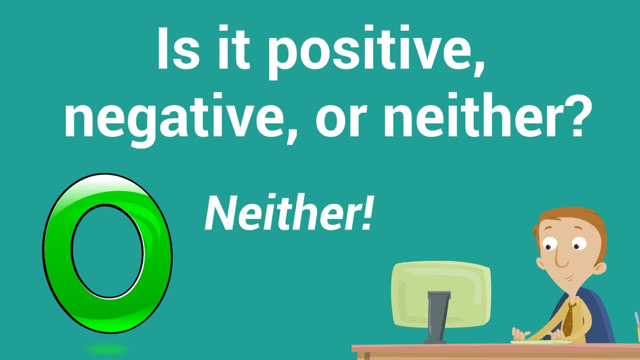 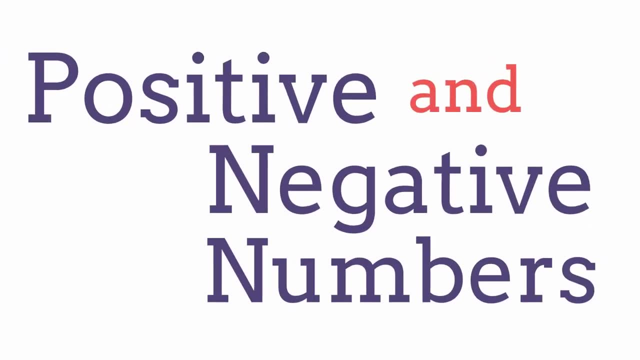 Do you remember? It's neither. Zero is its own thing. Wow, you really know your stuff. Well, that's what positive and negative numbers are. Keep a lookout for them, Especially those negative numbers. They are more rare to spot in the wild. 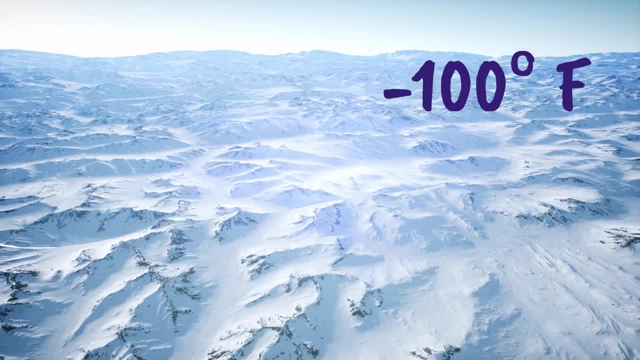 Thanks so much for learning about positive and negative numbers with me. I hope you had a wonderful time. If you had fun and haven't subscribed yet, it would be super cool if you clicked that subscribe button and clicked the notification bell so you get notified when I release new. 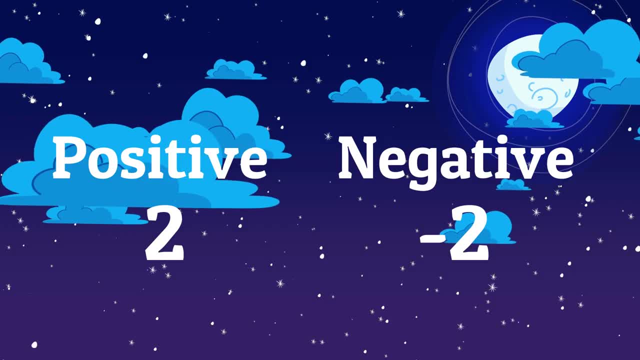 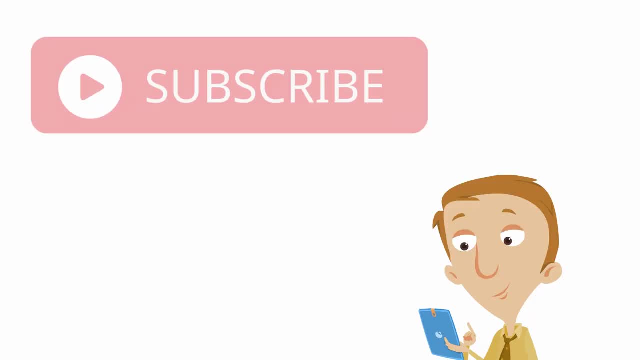 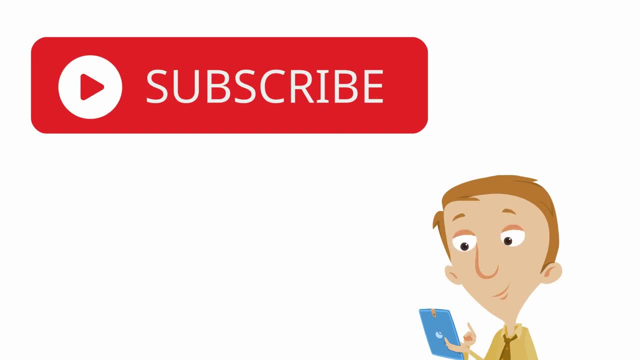 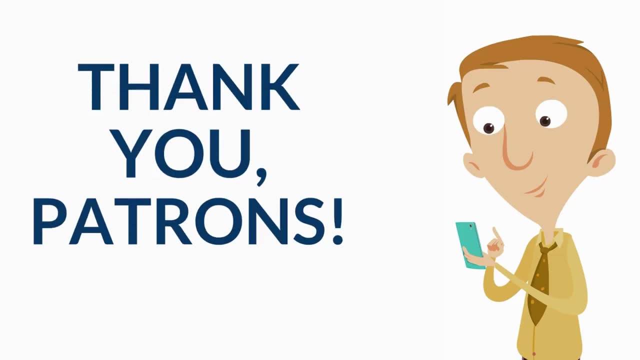 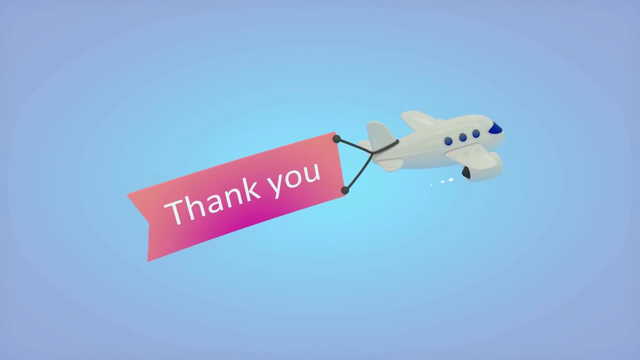 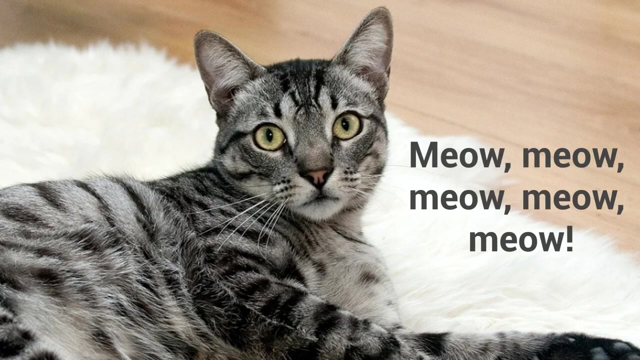 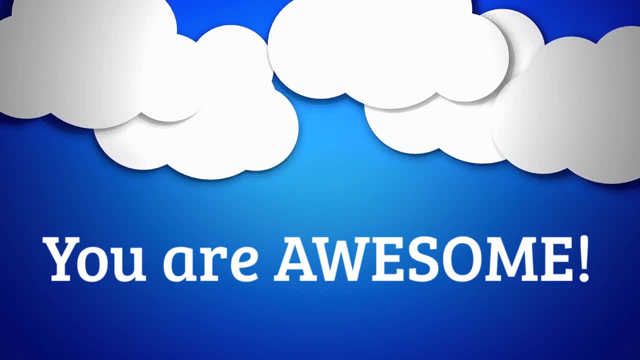 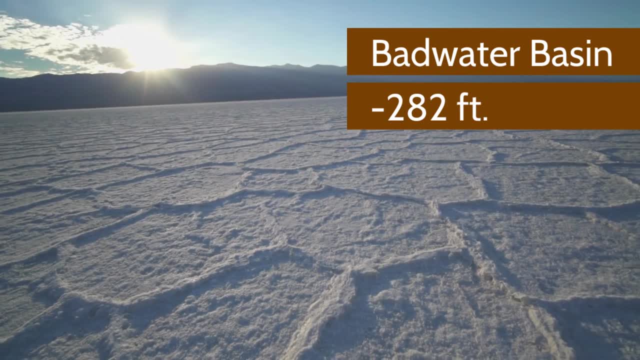 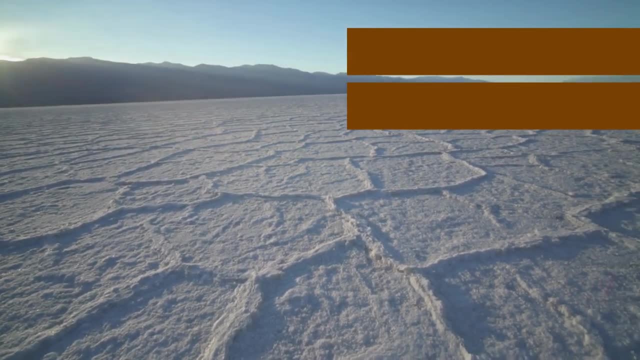 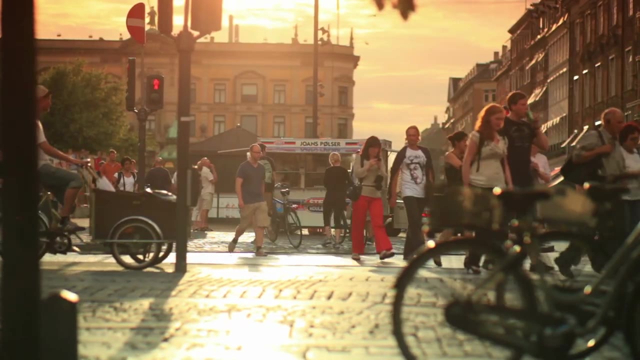 you are at negative 282 feet. That means you are 282 feet below sea level. Of course, elevations can be positive numbers and most places on land are above sea level. Where I live, I'm at 39 feet, meaning I'm 39 feet above sea level. 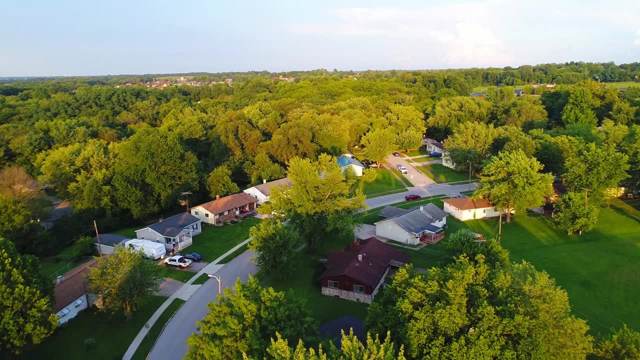 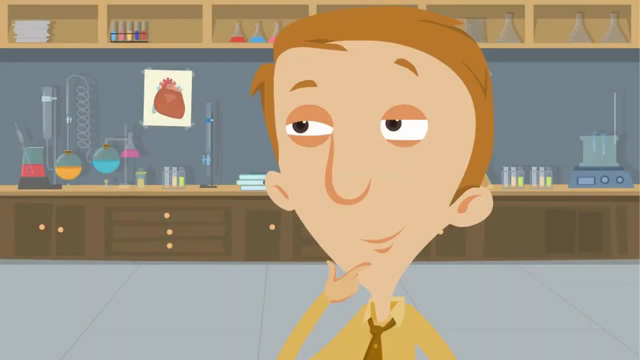 If you're curious about what the elevation is where you live, you can ask a parent or teacher. It's kind of fun to find out. Alright, the last example of negative numbers is if you owe someone money, Debt or money that's owed. 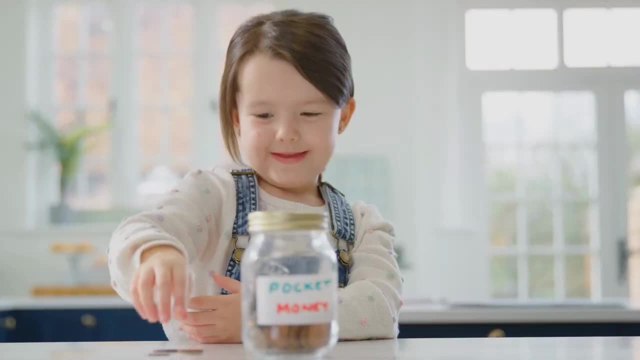 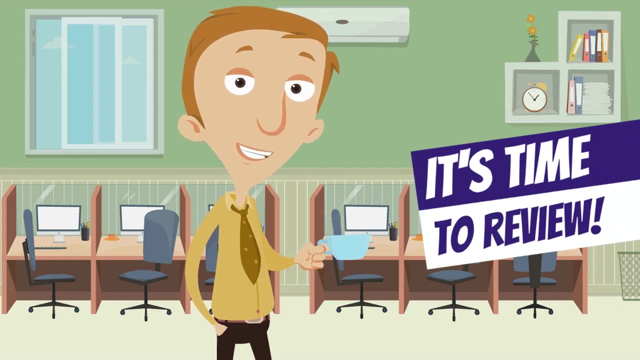 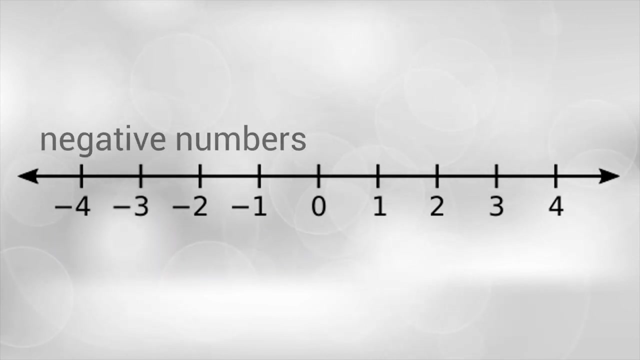 uses negative numbers. For money you get, you would use positive numbers. Okay, you know what It's time to review. It's time to review: Numbers below zero are called: Yeah, negative numbers. Great job. Numbers above zero are called. 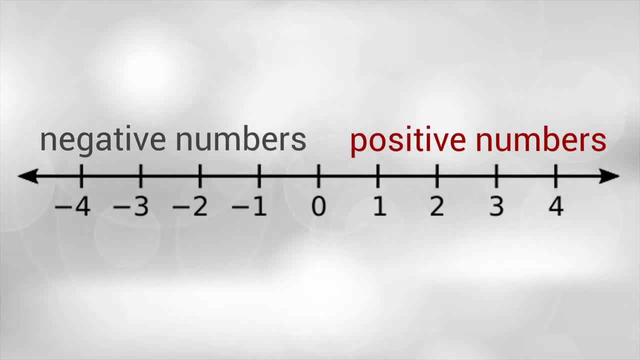 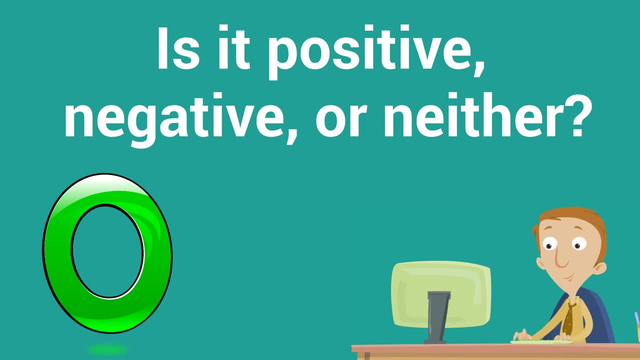 Got it. Positive numbers, Positive numbers, Awesome. And zero. is it positive, negative or neither? Do you remember, It's neither. Zero is its own thing. Wow, you really know your stuff Well, that's what positive and negative numbers are. 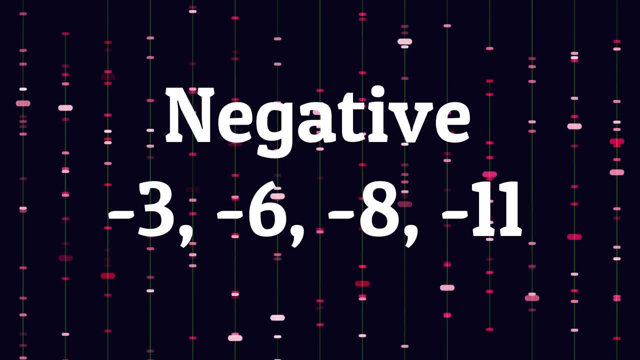 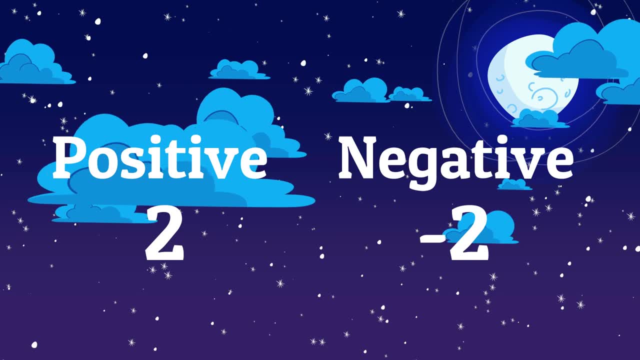 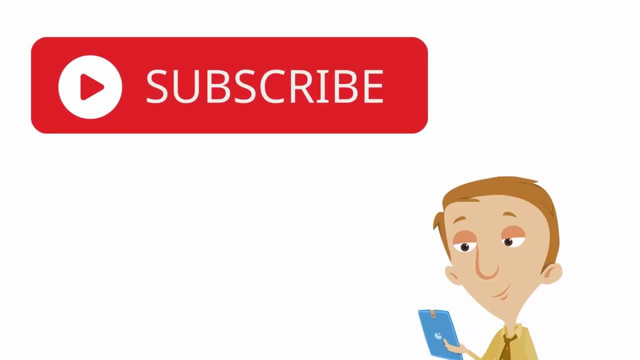 Keep a lookout for them, especially those negative numbers. They are more rare to spot in the wild. Thanks so much for learning about positive and negative numbers with me. I hope you had a wonderful time, If you had fun and haven't subscribed yet. 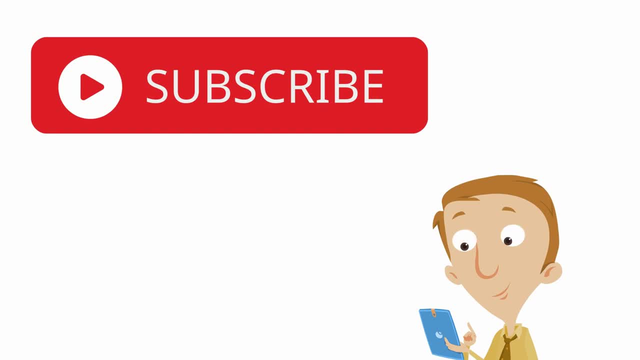 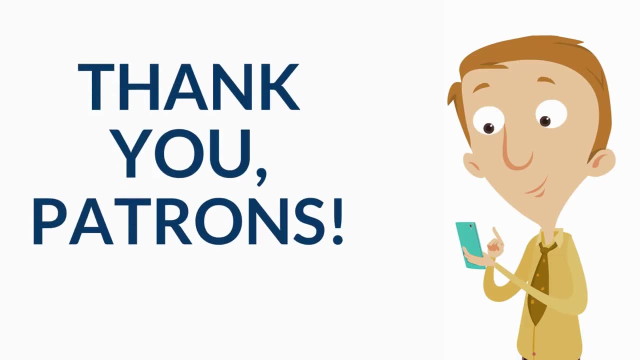 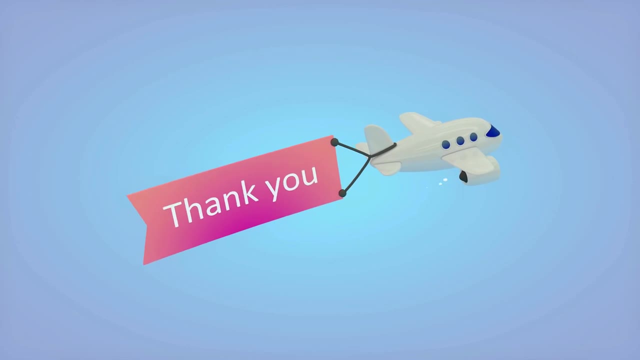 it would be super cool if you clicked that subscribe button and clicked the notification bell so you get notified when I release new videos. I want to give a special thank you to all of my patrons. It means so much to me And thank you for your support for watching. 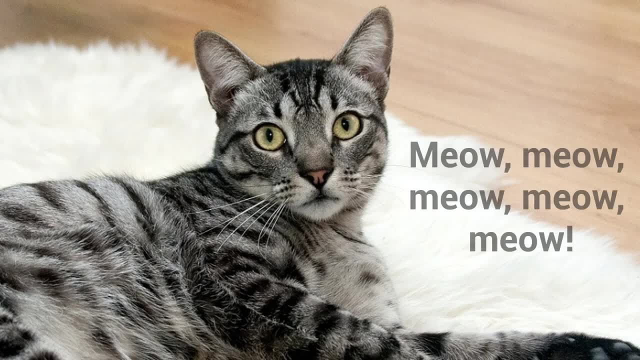 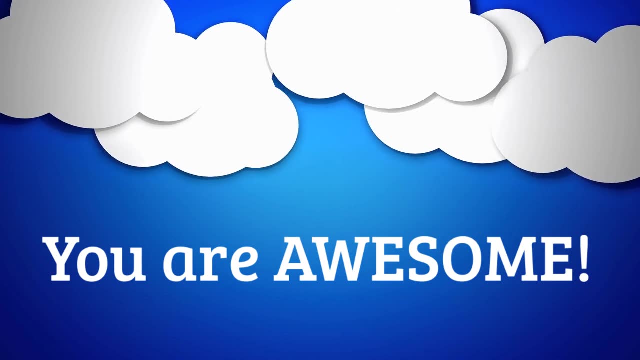 In the words of Mr Whiskers: Meow, meow, meow, meow, meow, Which I think means You are awesome. I'll see you next video.